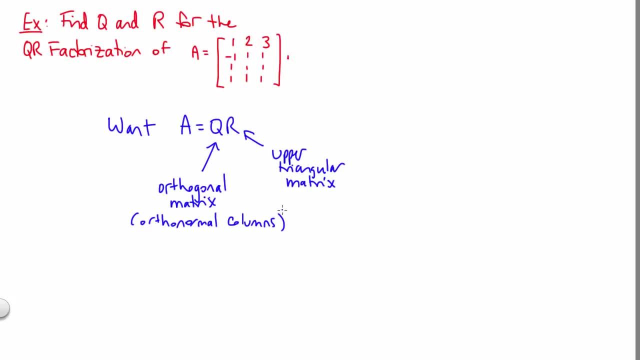 and R is an upper triangular matrix. Now, this will be possible whenever the columns of A are linearly independent. So our first step will be to take the columns of A and turn them into an orthonormal set, And we can do that using the Gram-Schmidt process. 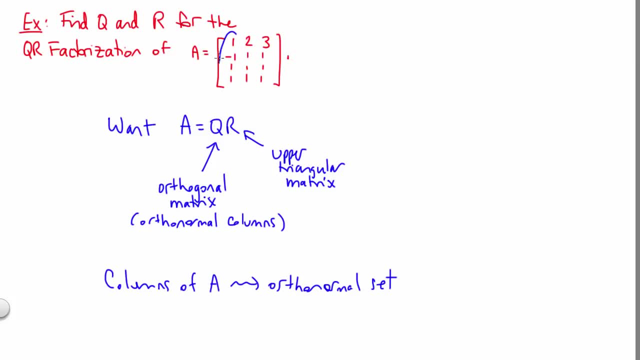 Now, in our previous video on the Gram-Schmidt process, we started off with this same set of three vectors here and we found the following orthogonal set, So I'm going to write here previous video. if you don't remember this example, you can look back at that video on the Gram-Schmidt process. 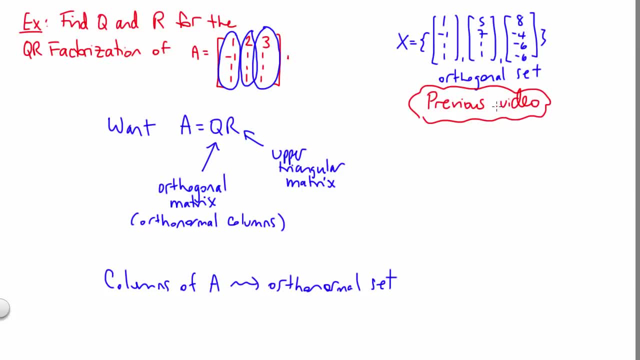 and figure out how we built this set X. We also mentioned in that video that we may want to simplify this last vector here. We could actually scale that by dividing each component through by 2. I think we should do that here, just to keep the numbers a little bit simpler. 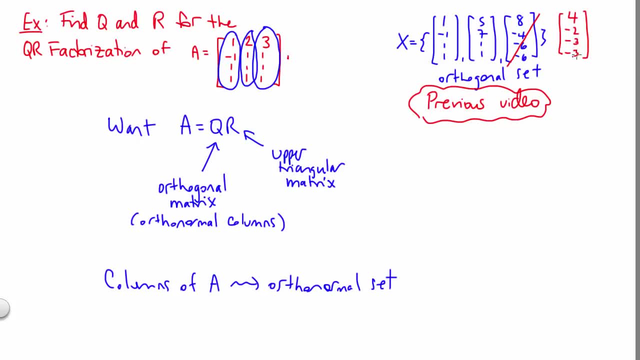 So this last vector is going to become 4, and So at this point we have turned the columns of A into an orthogonal set. But what we really want is an orthonormal set, So we're going to have to go through, divide each of these vectors, each of these three. 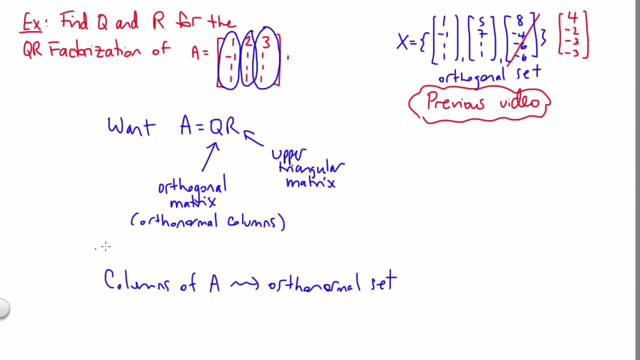 vectors by its length. So the length of that first vector is the square root of the sum of the components squared. So we'd have 1 squared plus negative, 1 squared plus 1 squared plus 1 squared. That gives us root 4, or in other words 2.. 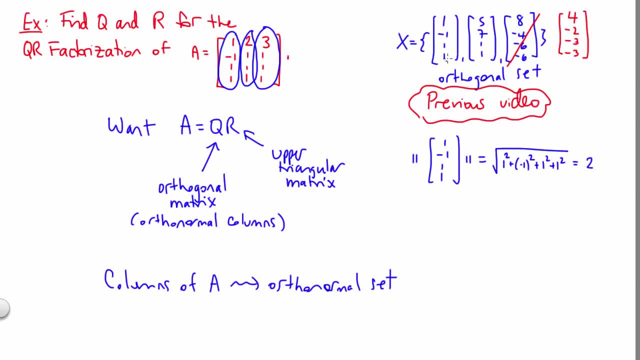 So to normalize that vector, we're going to go through and divide each of those components there through by 2.. So this is what our orthonormal set is going to look like: That first vector will be divided through by 2.. Okay, 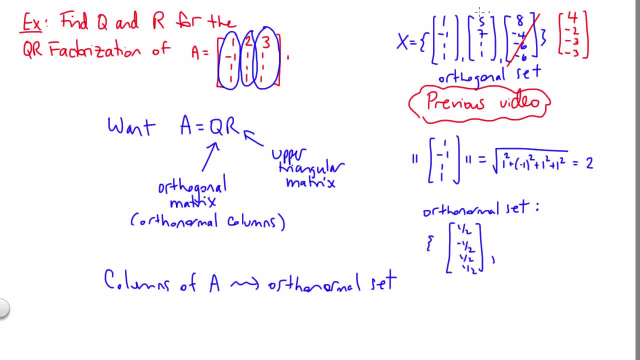 And in a similar way we can calculate the length of this second vector here to be root 76.. So the normalized version of this vector will look like this, And if we look at the simplified version of this third vector here, its length is root. 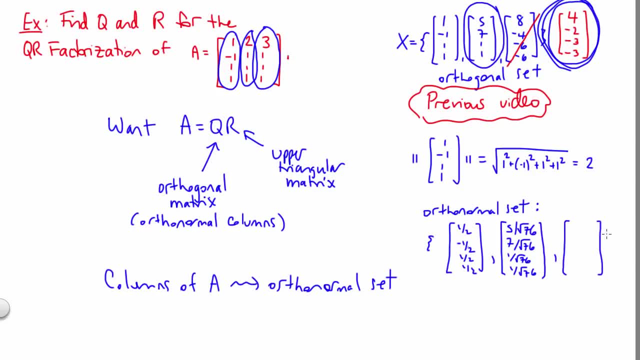 38.. So the normalized version of that vector will look like this. I'm not going to worry at this point about rationalizing any of these fractions or simplifying these fractions. We'll do that at the very end of the problem. At this point we're able to write down our matrix Q. 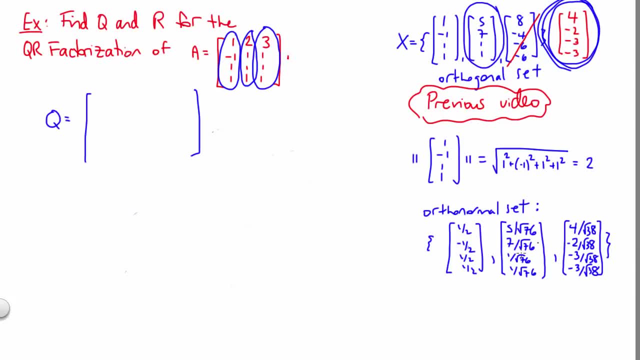 So the columns of Q will just consist of these vectors here that form our orthonormal set. Now let's figure out how to calculate R. Okay, Remember that we want A equal to QR, So the trick here will be to multiply on the left by Q transpose. 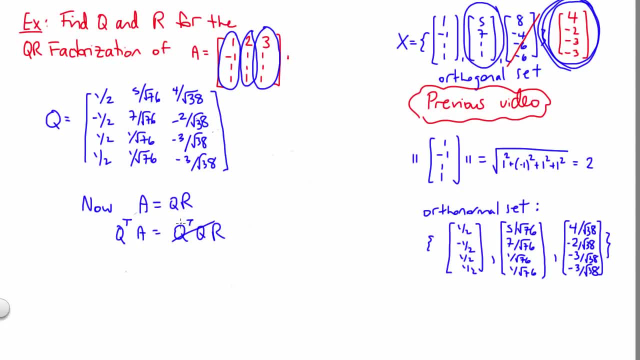 The reason that we do that is that Q is an orthogonal matrix, so Q transpose, Q is guaranteed to equal the identity matrix. So, in other words, on the right side we've got IR, which just gives us the matrix R. So we've got this little formula here that reminds us how to calculate R. 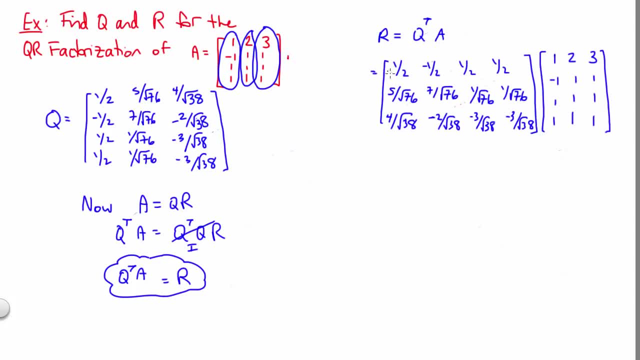 I think I'll circle the rows of Q transpose here in the columns of A, just to make this calculation go a little bit more smoothly, because there are a lot of roots in this expression. So the nice thing about this calculation is that when we grab the first row here, everything's. 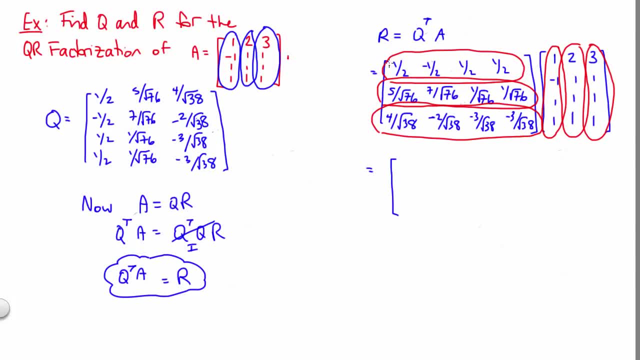 over 2.. So we really just need to pay attention to the numerator. here We're getting 1 times 1 plus minus 1 squared. plus 1 squared plus 1 squared gives us 4.. So it's really 4 over 2.. 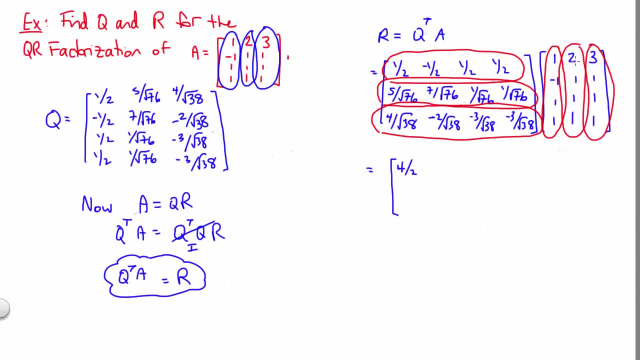 Moving over to the second entry again, if we just look at the numerators- 1 times 2 plus minus 1 times 1 plus 1 times 1 plus 1 times 1, that's going to give us 3.. 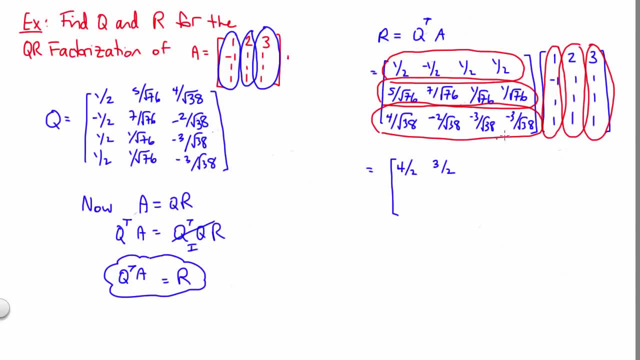 So that's 3 over 2.. And then finally, in the top right here, we've got 4.. We've got 4 over 2.. So we'll simplify these entries in a minute. Moving into the second row, we've got 0 over root 76.. 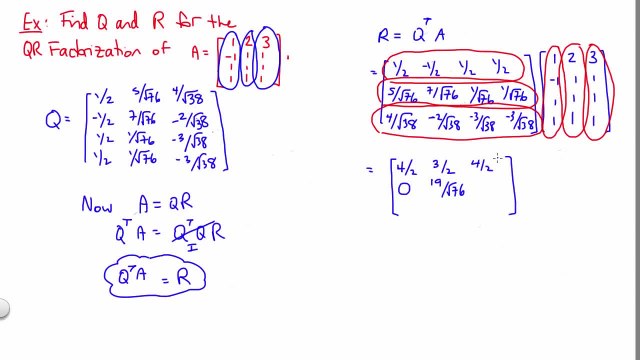 Then we've got 19 over root 76. And for the third entry, 24 over root 76.. OK, now, moving into the bottom row, we've got 0,, 0, and then finally, 4 over root 38.. 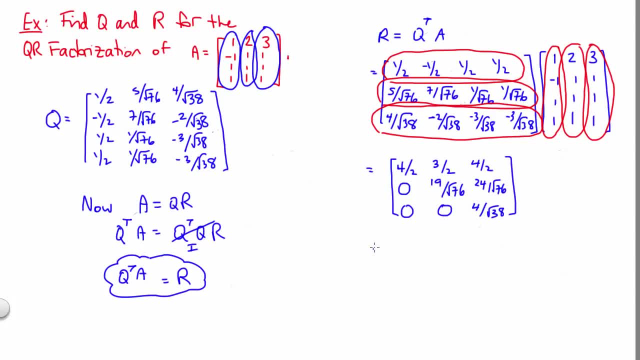 Now that we've found q and r, let's think about simplifying the entries in these matrices. Top row comes out to 2, 3 halves 2.. In the middle row we've got 2.. In the middle row, if we simplify this fraction here, 19 over root 76, we can call that root. 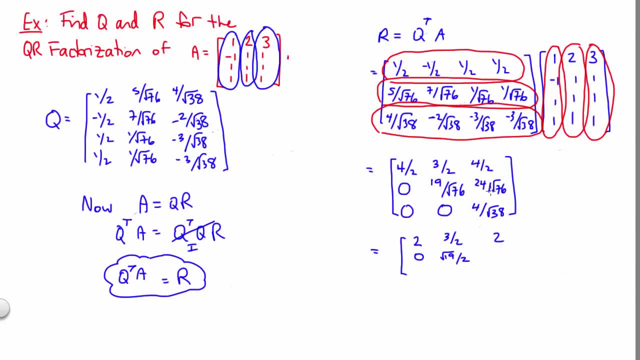 19 over 2.. And in this third entry here this guy's going to simplify to 12 root 19 over 19.. And then finally, in the bottom row here, 4 over root 38 is going to simplify to 2 root. 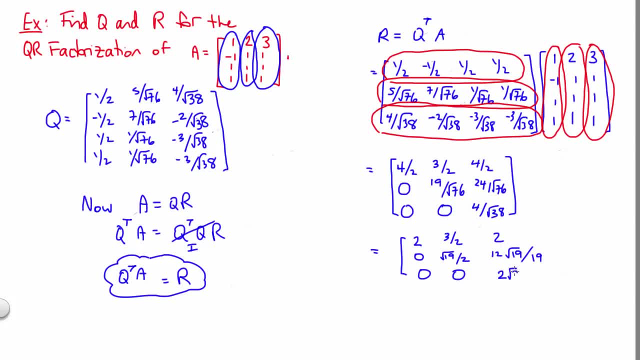 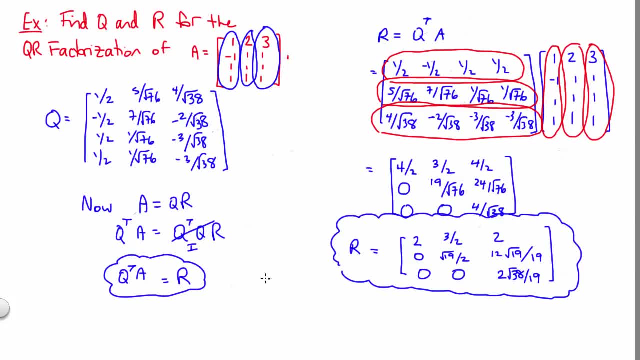 That's 1 half of our final answer, And very last thing we'll need to do is just simplify our matrix q So we can refer back to the matrix q that we had written down earlier in the problem, And we now just need to simplify this for our final answer.